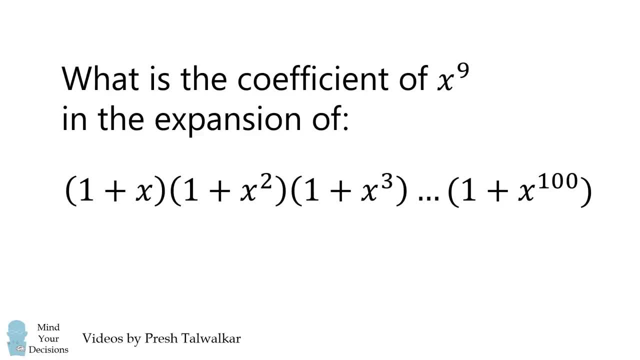 all the way until the last term of 1 plus x to the power of 100.. This was asked on the JEE Advanced Exam, which is a test used for admission into India's prestigious IIT colleges. Pause the video if you'd like to give it a try and when you're ready. 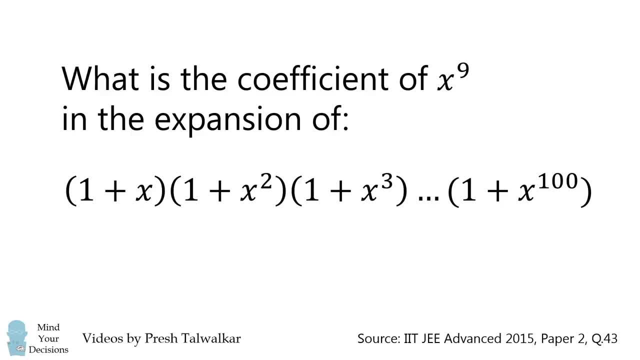 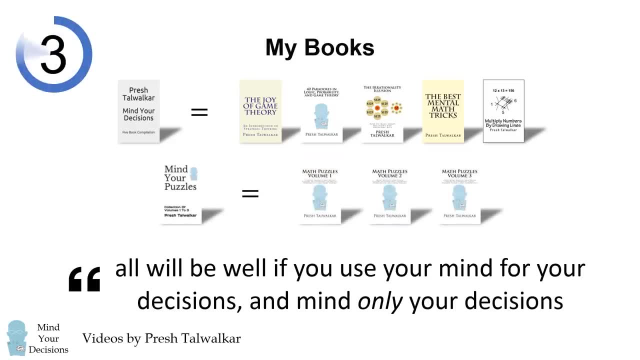 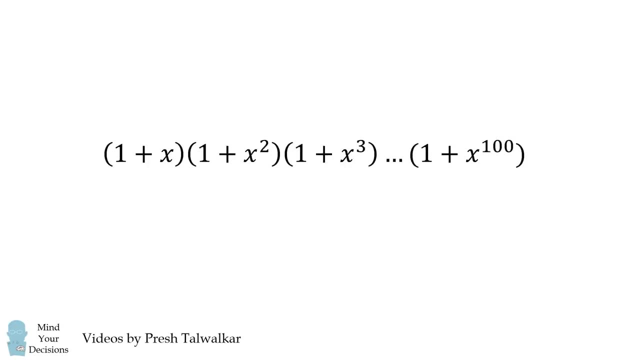 keep watching to learn how to solve this problem. Let's analyze this binomial product. Consider the term 1 plus x to the power of 10.. What happens if we multiply x to the power of 10 by ones? in all of the other binomial terms, We'll end up with x to the power of 10.. 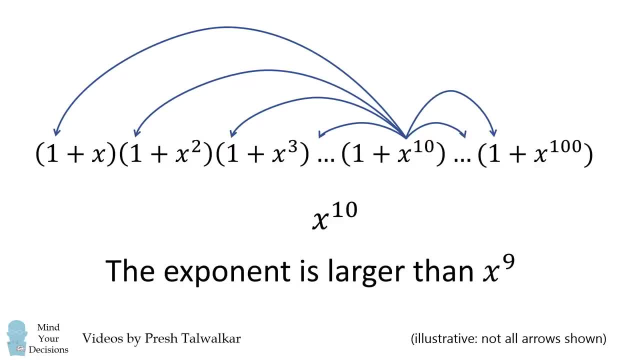 Notice, the exponent is larger than x to the power of 9, so this will not contribute to the coefficient of x to the power of 9.. Similarly, if we have 1 plus x to the power of k, where k is greater than 9,. 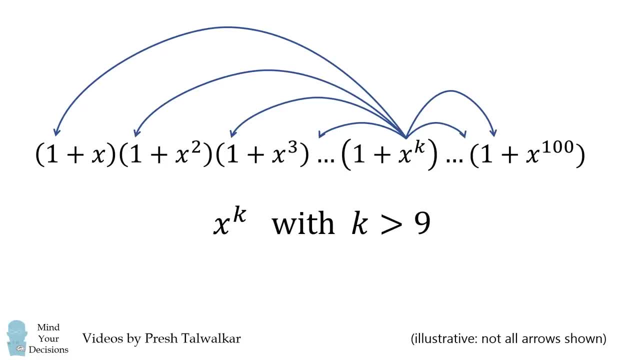 if we multiply this by all of the one terms in all of the other binomials, we'll end up with a term that is an exponent that's larger than 1, and the exponent that is larger than x than x to the power of 9.. So we don't need to focus on any of these terms to get the coefficient. 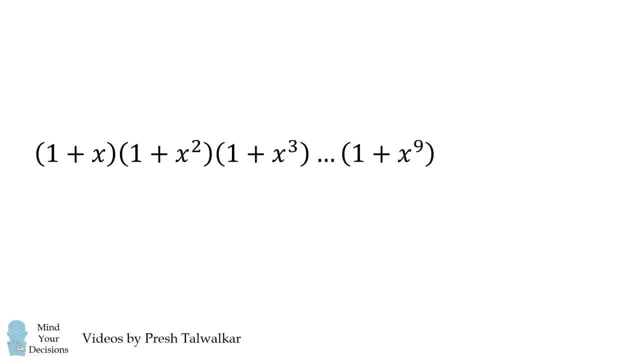 of x to the power of 9.. We'll only go up to 1 plus x to the power of 9, and then we'll distribute this term with all the other ones in all of the other binomials. So let's analyze this binomial. 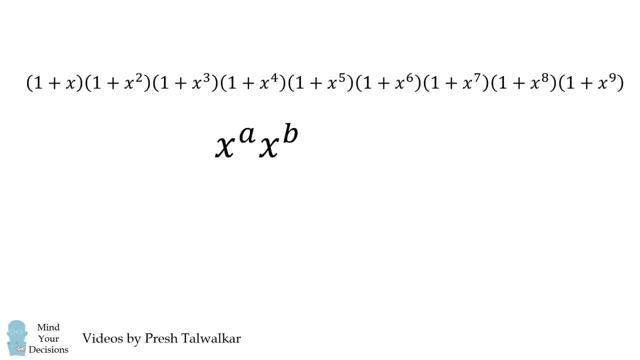 product. We'll recall an exponent rule: x to the power of a multiplied by x to the power of b is equal to x to the power of a plus b. We're therefore going to count the ways that the exponents sum to 9, and the exponents are the numbers from 1 to 9.. We'll then multiply the result by ones from all. 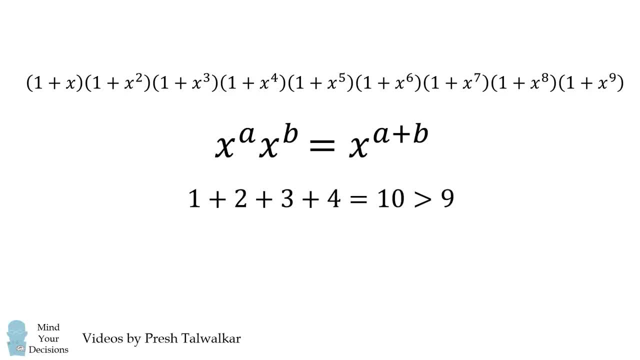 of the other binomials in the product. Now here's a simple observation: 1 plus 2 plus 3 plus 4 is equal to 10, and that's greater than 9.. So we can only have three, two or one terms in the product. 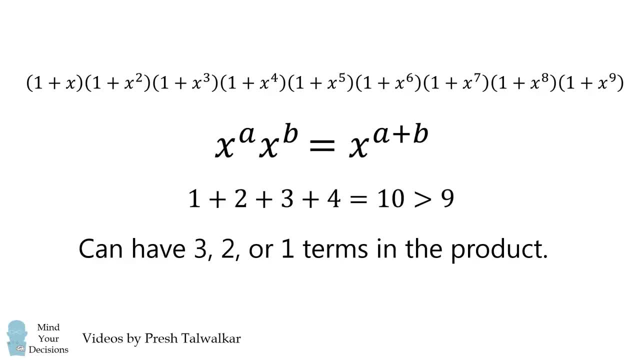 If we have four terms, we're going to get to an exponent that's larger than 9.. So let's enumerate the ways. If we have one term, we just have x to the power of 9.. For two terms, we just have x to the power of 9..